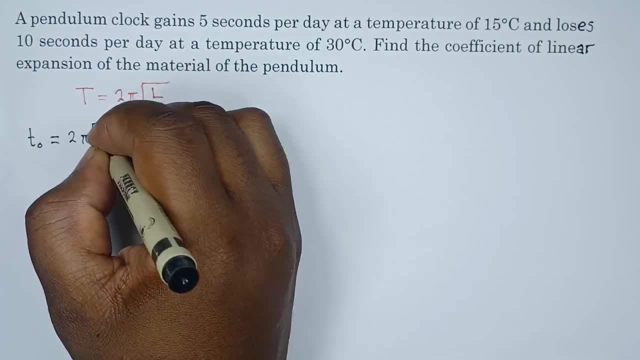 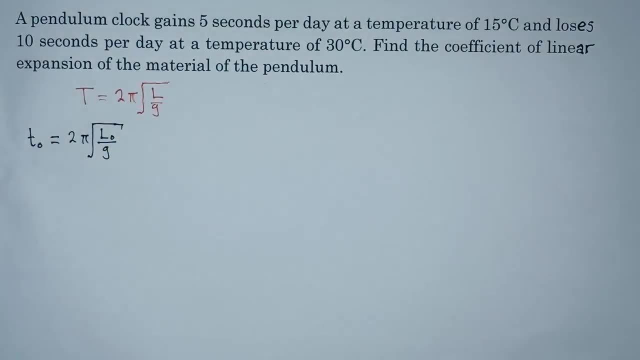 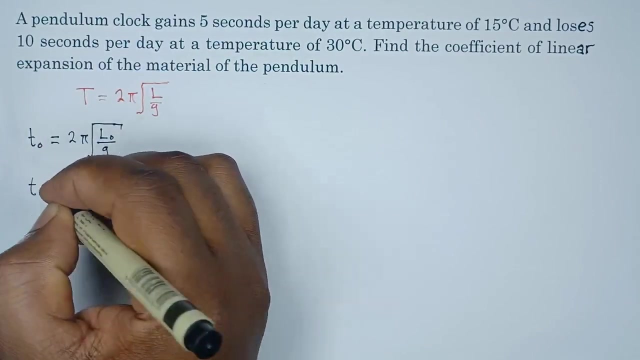 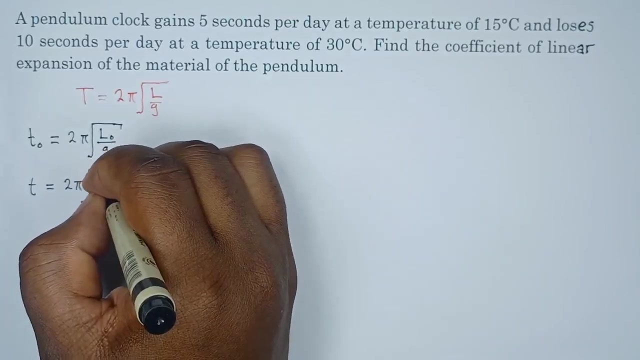 root of L, The square root of the initial length over G, Like that Also. at the same time we're going to say t final now. So t final is equal to 2 pi square root of L over G, According to how we find the linear expansion Okay. 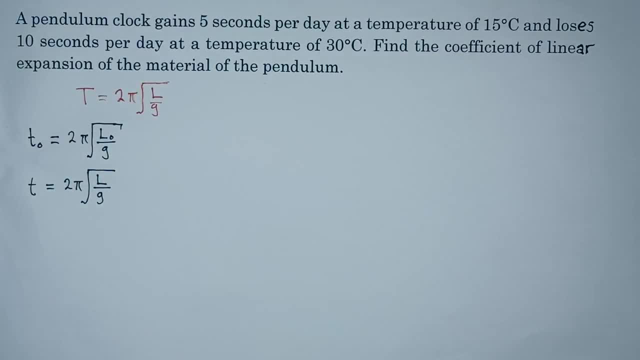 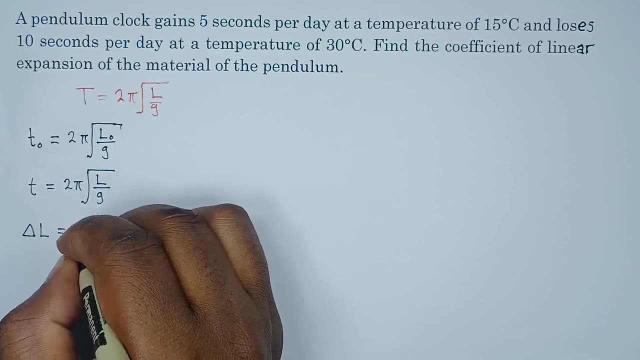 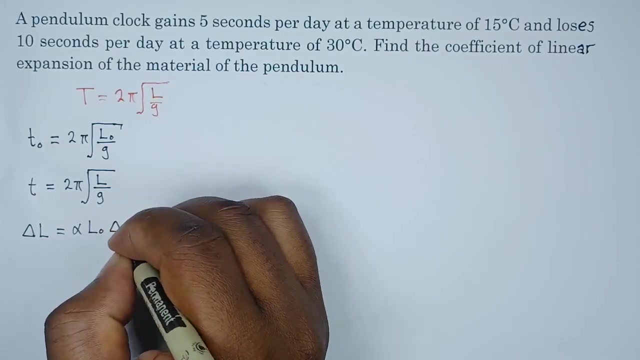 Okay, Let's take a look at the linear expansion of the material. So we're going to note that the change in the length is equal to alpha, which is the linear expansion multiplied by the initial length, multiplied by the change in temperature. 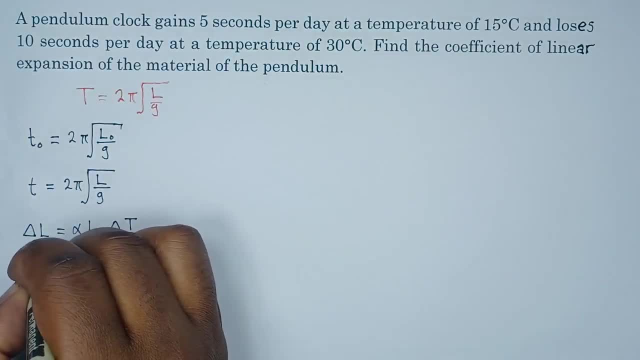 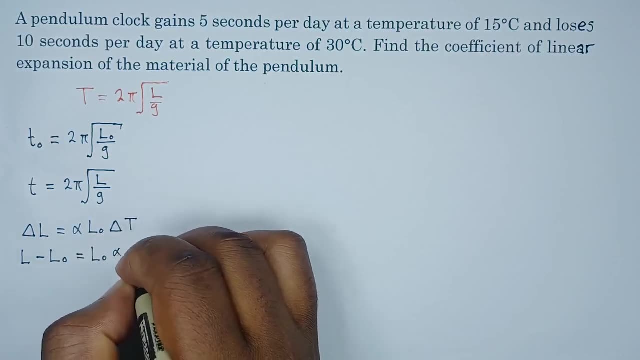 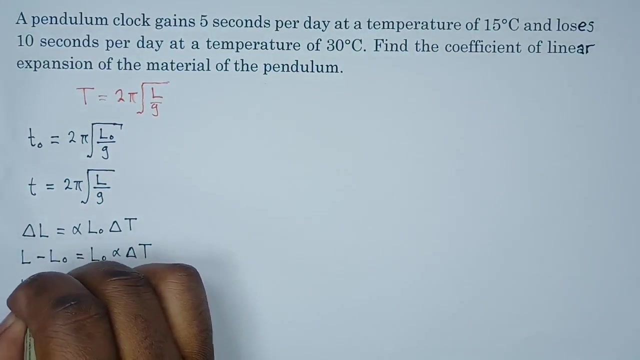 So the change in the length is simply L minus L initial, which is equal to L initial. alpha times the change in temperature: Okay, alpha times the change in temperature. then let's make L the subject here. so L will simply be equals to L. 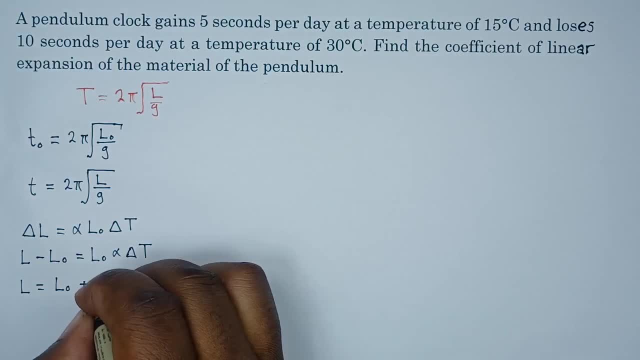 naught, plus it's a negative, becomes a plus L naught alpha change in temperature. so we can factor out L naught here. so L will be equals to L naught open bracket one plus alpha change in temperature, like that. so now that we have this expression, that we have here, 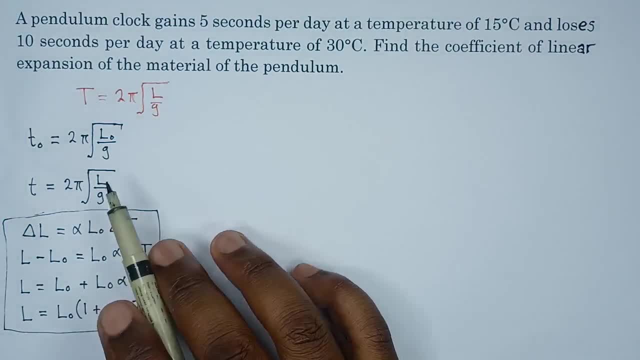 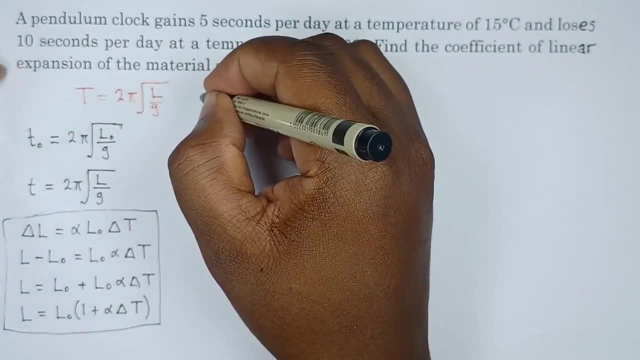 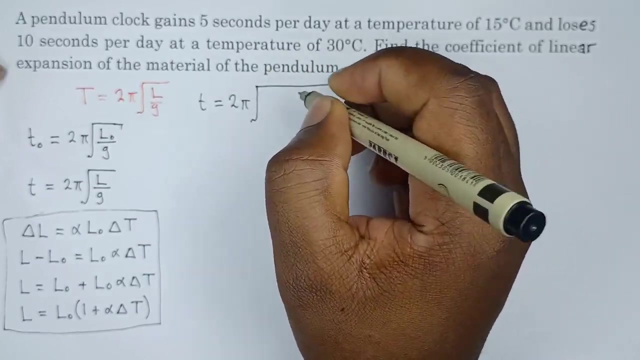 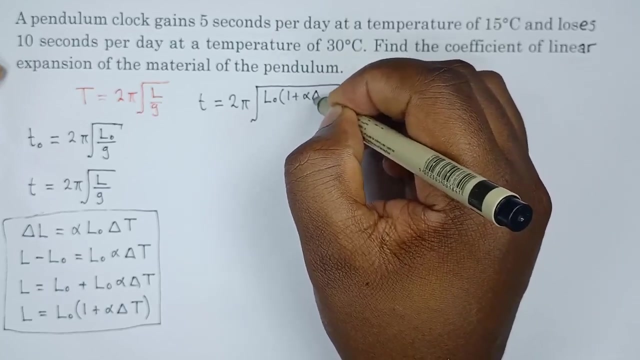 we are going to substitute here where we have L, so if we bring it here T, remember this one is T initial, that one is okay, so this one will have. T is equals to two pi square root of our initial open bracket, one plus alpha change in temperature. 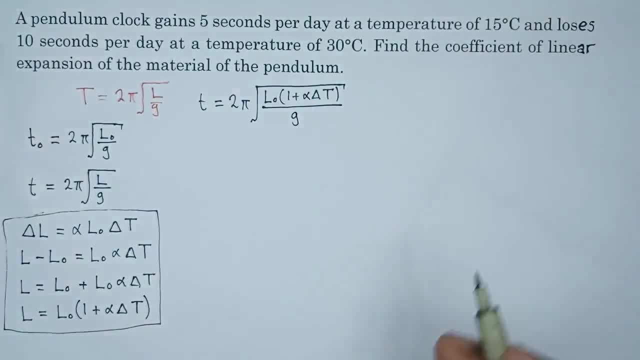 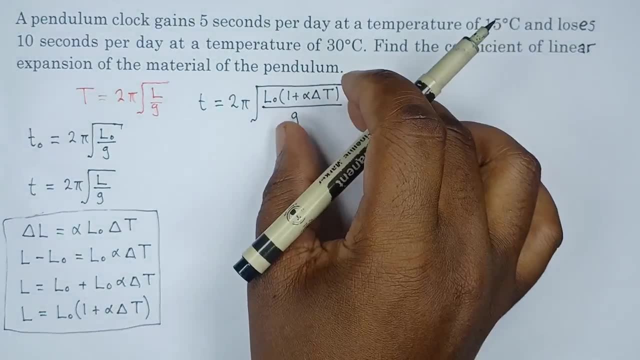 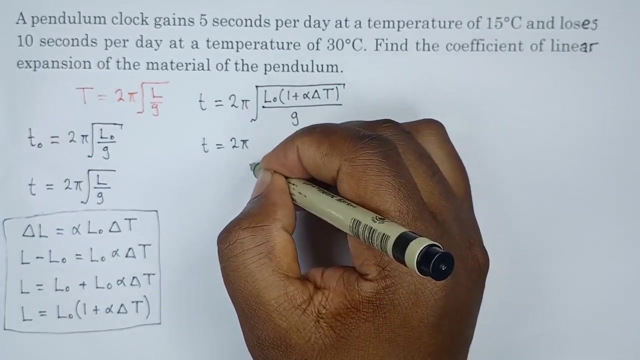 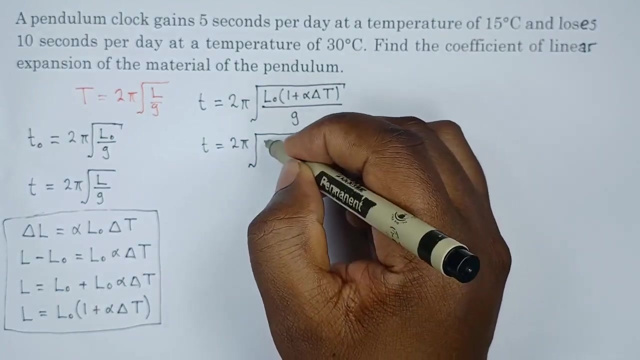 everything is over over G that. so the next thing we can do now is, for this same part that we have, we're going to split it inside the square root. there we can have it, as T is equals to two pi, so we have the square root of. so what the L naught and G. so we have L naught over G. 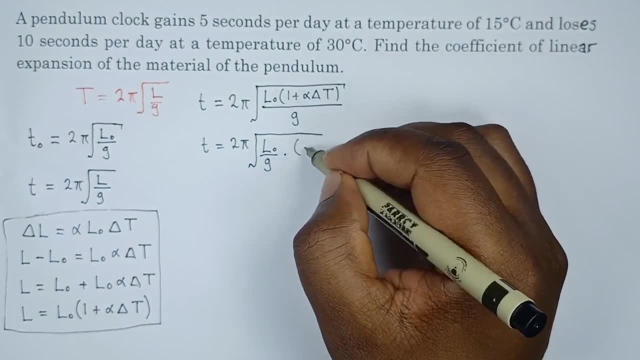 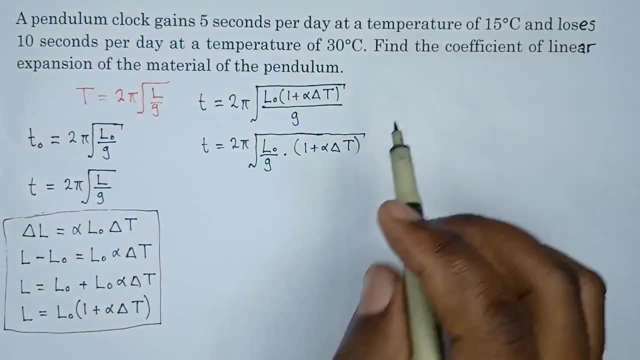 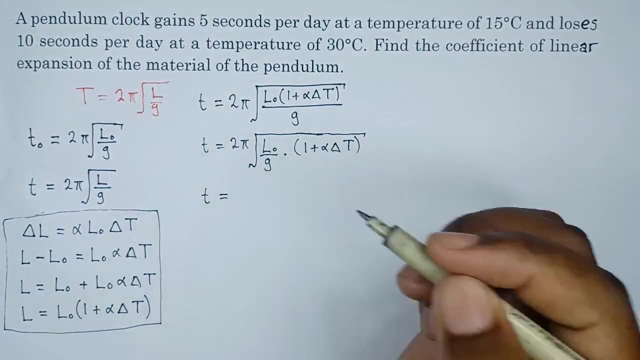 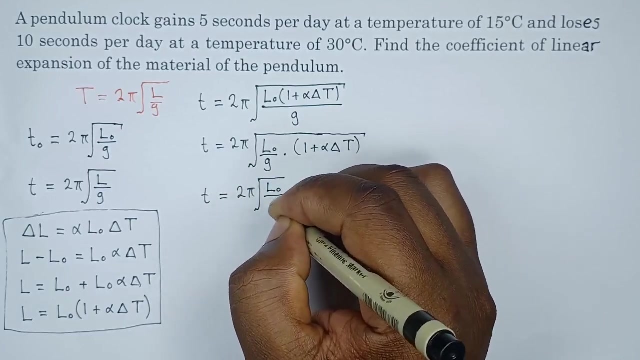 remember, everything is inside the square root multiplied by one plus alpha. change in T, like that. so since the two are multiplying inside the square root, we can split the squared root now. so we have: T is equals to 2 pi. the first square root will be L0 over G. 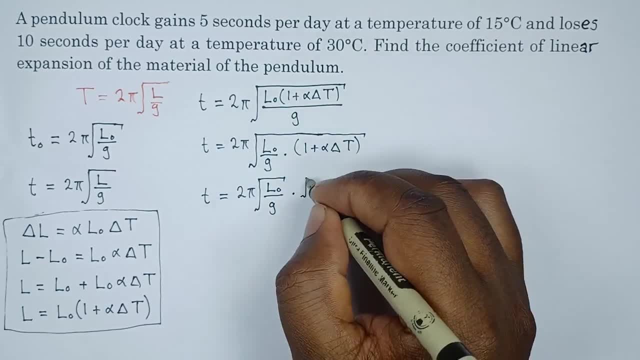 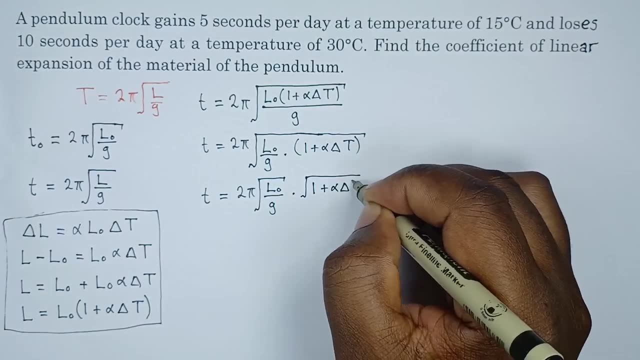 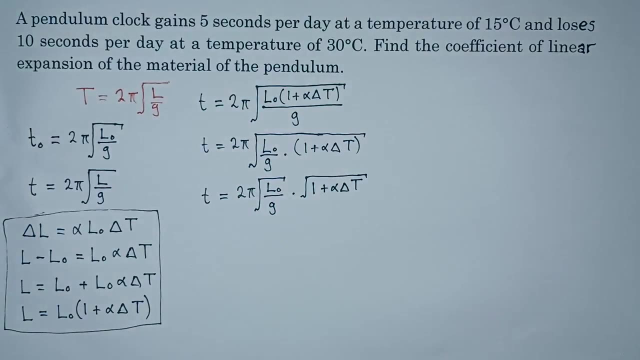 multiplied by the square root of this, which is, so we just split the square root- 1 plus alpha. tangent T, remember alpha is the linear expansion of the material. so now that we have this expression, we can clearly see that this part here is the same as T0. 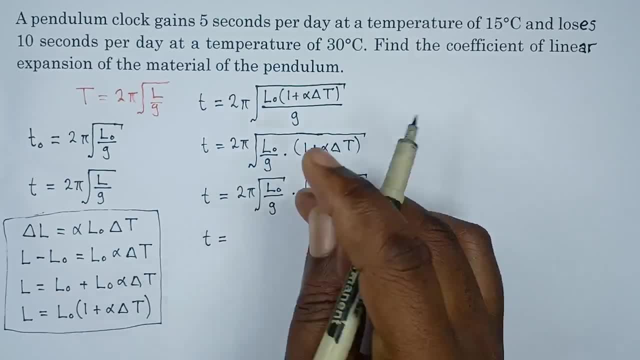 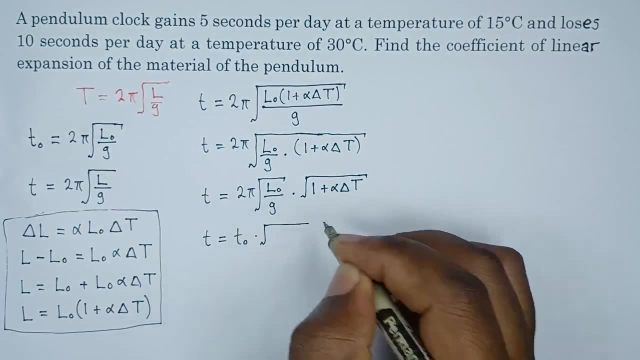 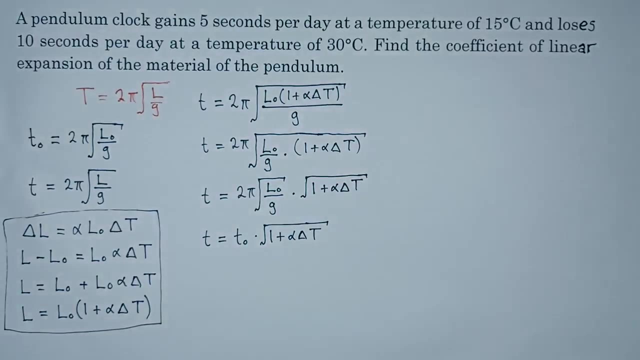 so T equals to. we replace this equation with that and we get T0 multiplied by the square root of 1 plus alpha T. so now there's a concept I'd like us to remember from Binomial Theorem. so now there's a concept I'd like us to remember from Binomial Theorem. 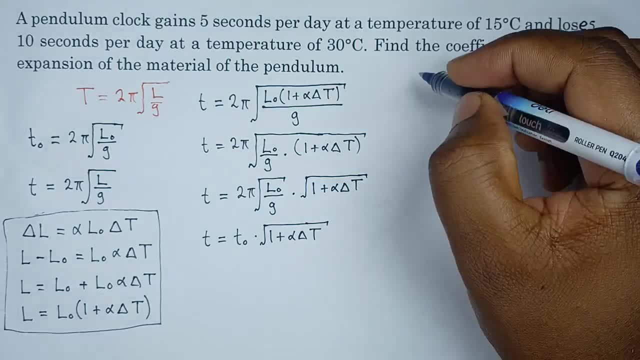 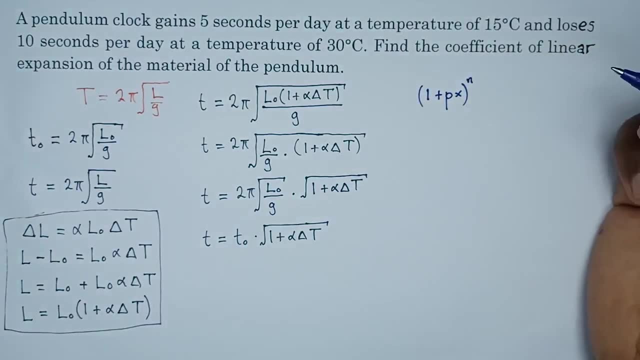 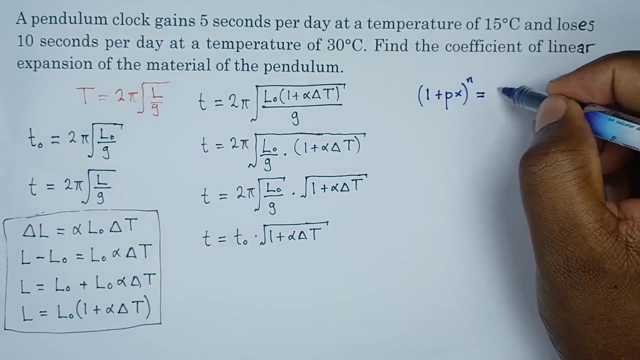 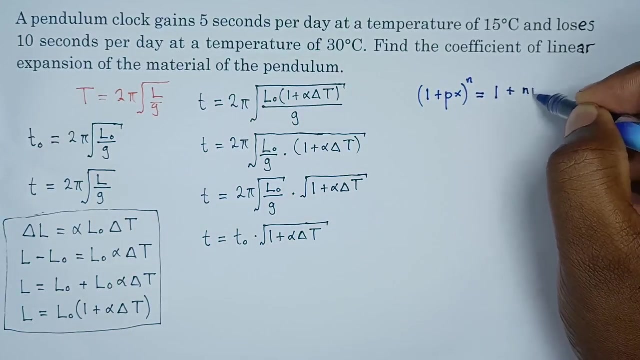 expansion. so according to binomial expansion, if you have the expression 1 plus px, for example, raised to the power n, so n can be a negative number, n can be a fraction, n can be anything. so the expansion for the first two terms will be given by 1 plus the product of n, p and x. this is just from binomial expansion. 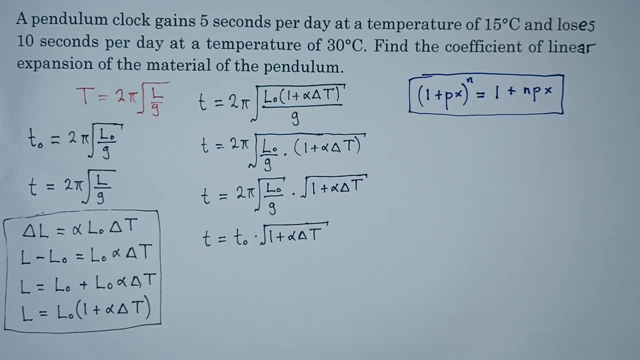 in the bracket, tillゞ. so I want to use this similar concept, what we have here. so if we write the statement, if we were right, the square root will have T is equals to T0. multiplied by this will become one plus alpha, random temperature raised to the power half. so remember, square is power half. let's use a similar concept. that we have here. we say T is the light constant. I'm just going toflow an old Landmass argument. as you transform the Sternin and theозиomonową period by I will need T plus N, so number of عتamperature to do. that means I should be able to apply the Union equation that say: n to the power Half, because, remember, square root, its power of half. let's use the, the schooling of a concept. have here we said II, and the 5 separitenlegable 표현 of this requirement is called energized as part of causal, because the co-operation of this equation literally can be appreciated. because then, if we've seen the 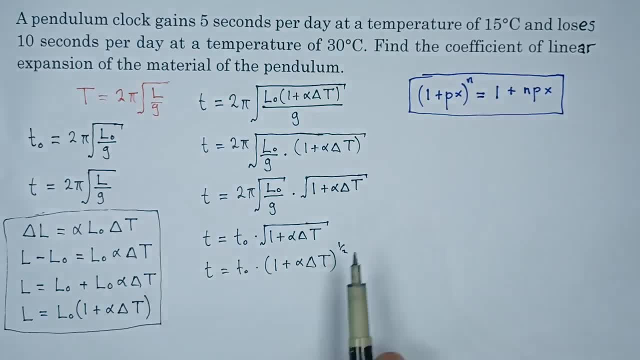 the first time is 1. then we multiply n, p and x. this time around. the first time is still 1. then we multiply half alpha and change in temperature, so T will be equals to T. naught using the binomial expansion, what we want to have will seem to be 1 plus half is as good as the n. 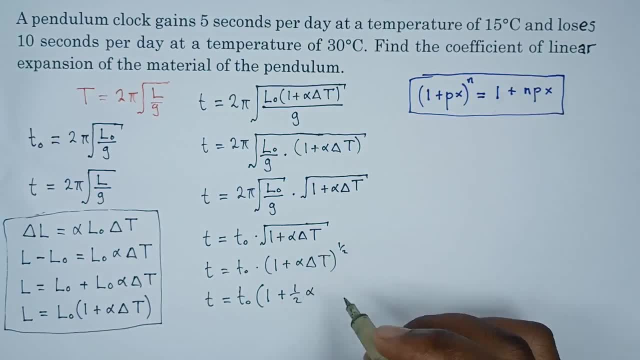 multiplied by alpha and the change in temperature, like that. so this is the expression that we have now. now to this expression. this is what I want to do. it we still have to manipulate it. let's expand. so this T naught should expand. so what we want to get will be: T is equals to, so T naught times 1. 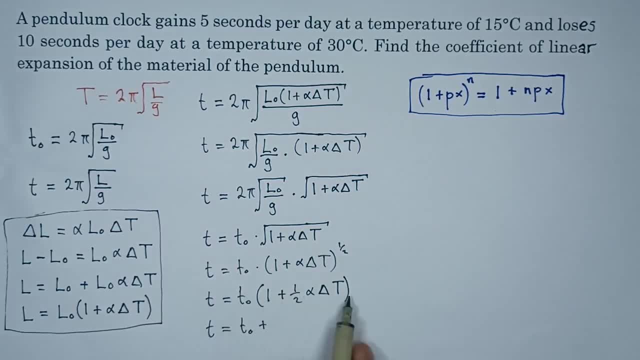 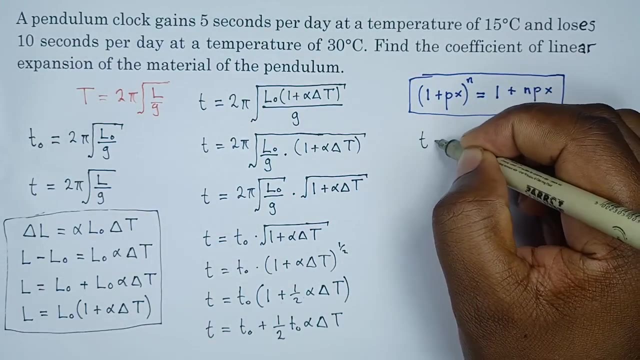 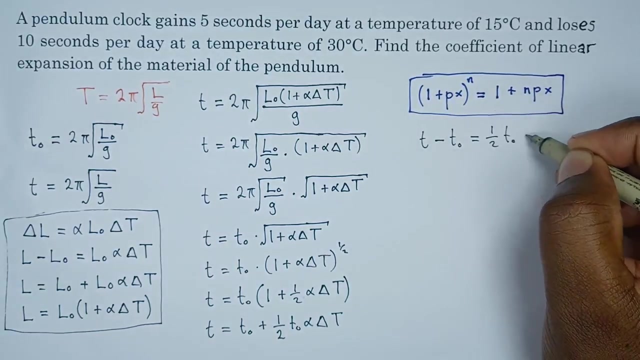 from which T naught. like that T naught times this expression, we'll have half T naught alpha change in temperature. let's push the T naught to the other side, so we get T minus T naught is equals to half T naught alpha. 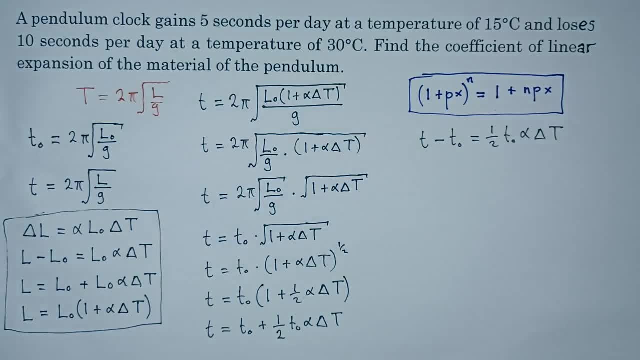 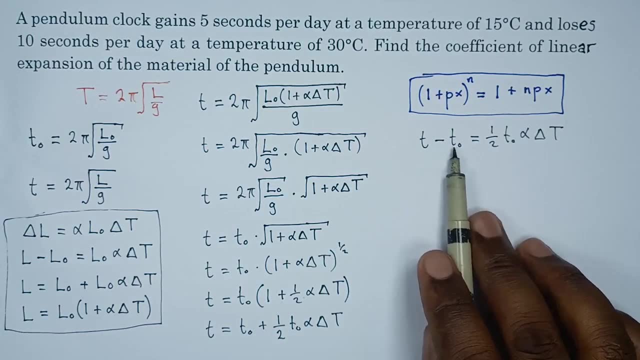 change in temperature like that. okay, so now we want to get rid of this T naught, but before we do that, we want to get rid of this T naught. so we want to get rid of this T naught, but before we do that, we know that this is a change in time. 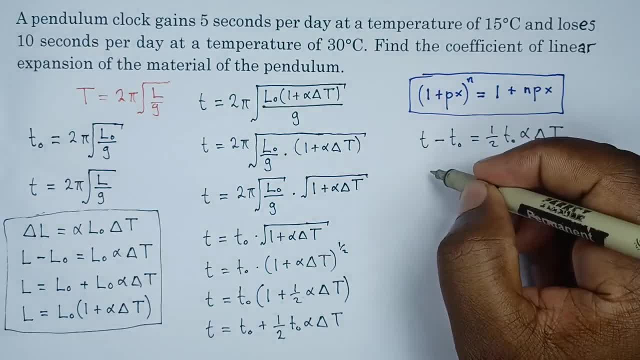 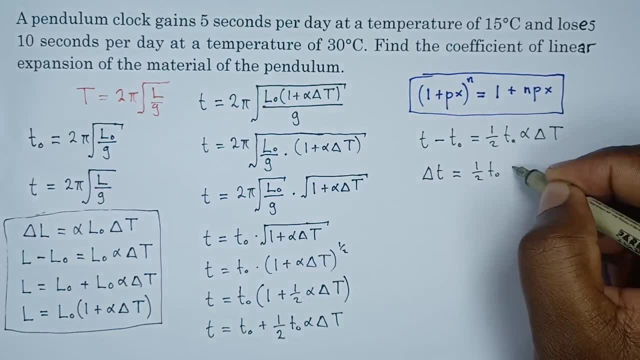 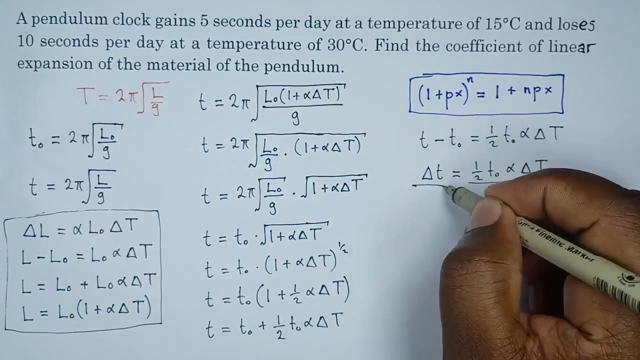 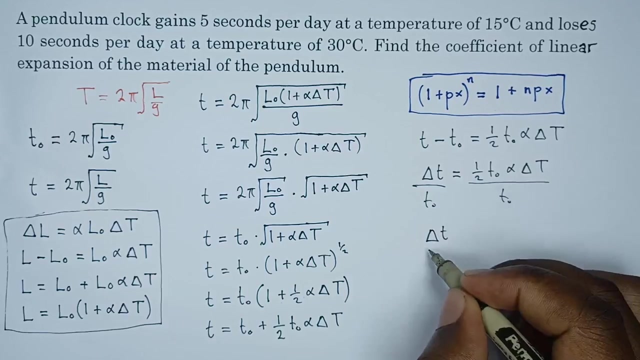 that is T final minus T initial. so this is just a change in time. so is equals to half T naught. alpha change in temperature. we divide both sides by T naught. we divide T naught by T naught what we get. so the change in time. 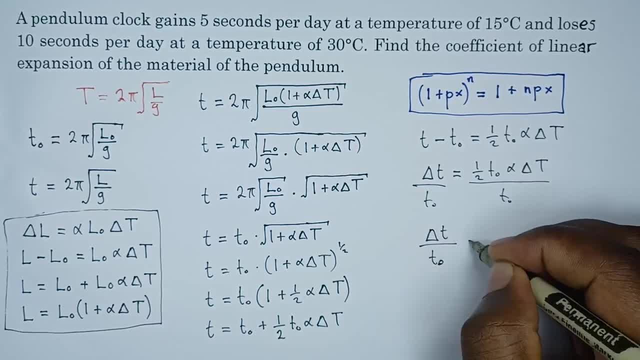 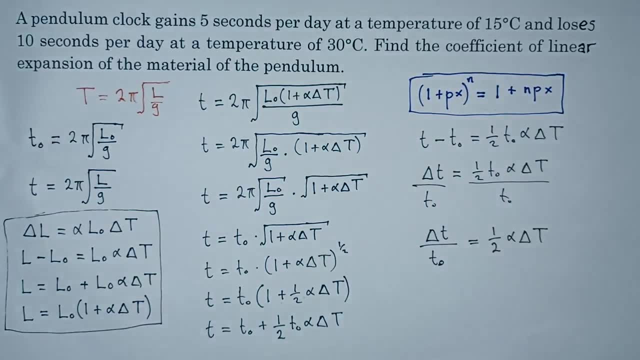 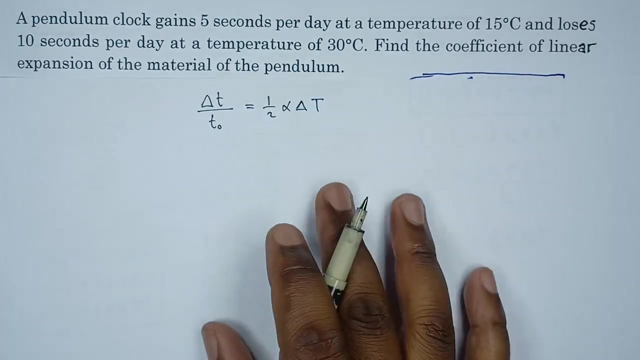 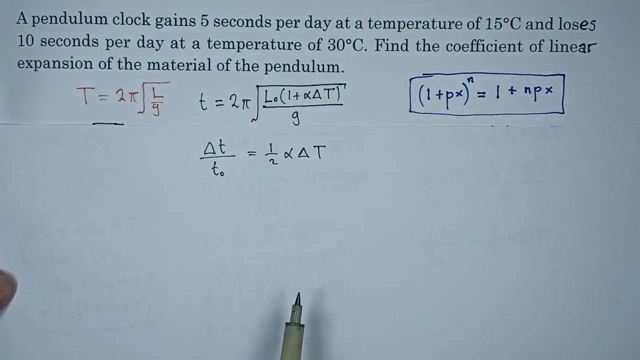 over T naught. t naught initial time is equals to half alpha changing temperature. okay, so this is the expression that we are going to use to find out everything that we are looking for. so, to start with, so this is the expression that we have. so we have two statements here, or two. 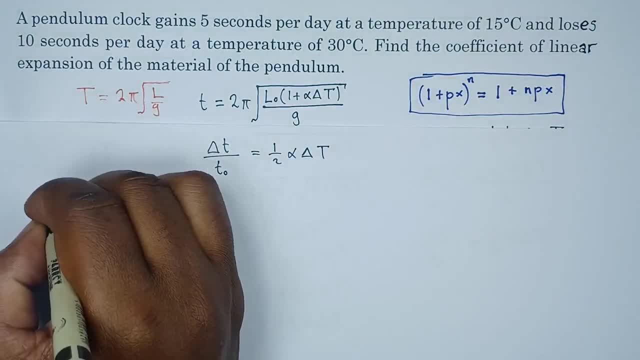 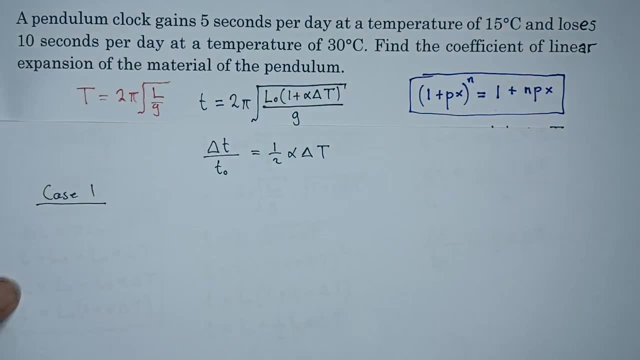 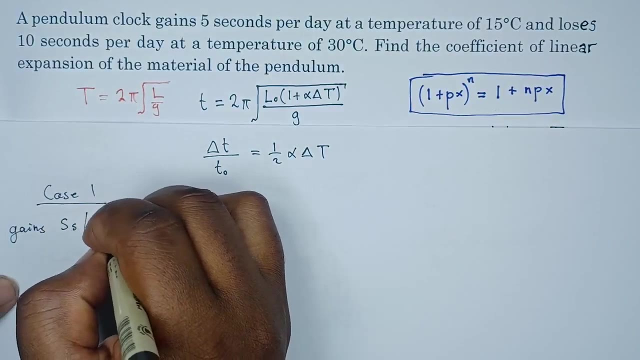 parts, let's do it separately. so let's start with case one. I'll call them case one and case two. so for case one, what is happening? a clock gains five seconds a day. so gains five seconds a day, okay, at a temperature? at a temperature of 15. 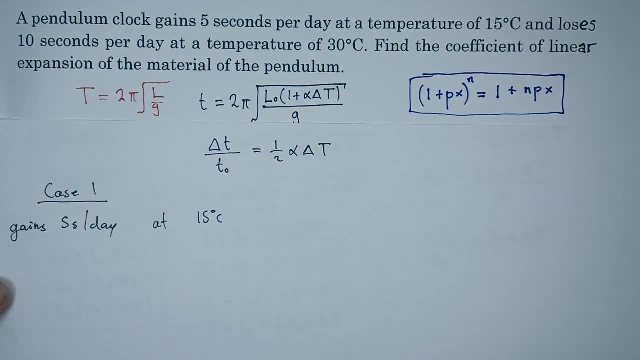 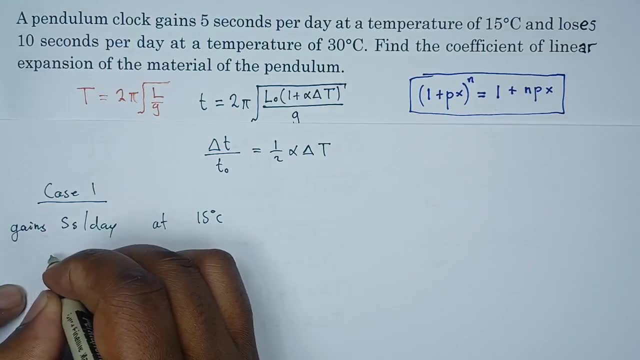 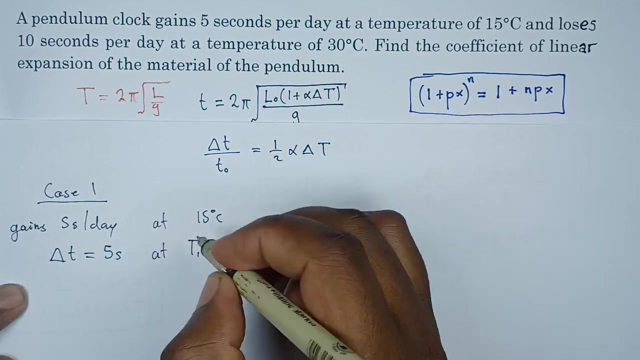 degrees Celsius. so if that's the case, let's see what happens. so what does this mean for us? it means that the change in time and in time will be five seconds at a temperature, at the temperature of 15 degrees Celsius. now we're going to call this the initial. 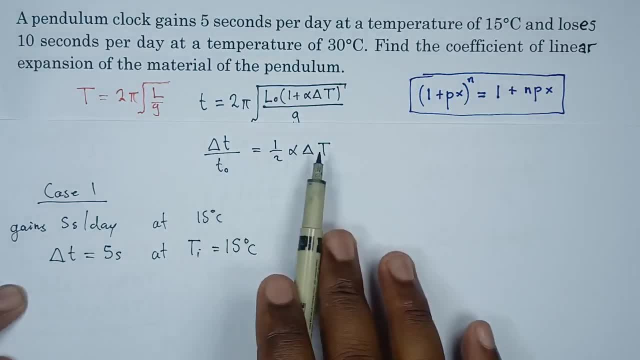 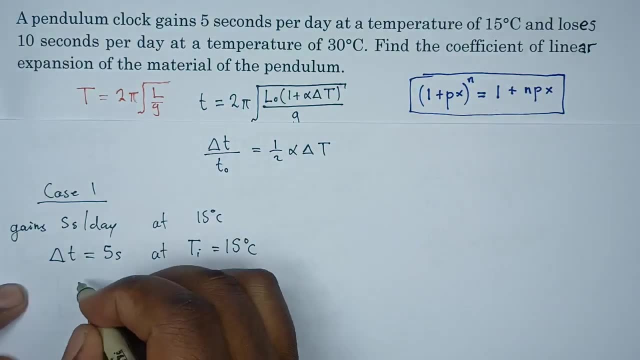 temperature. so if this is the case, using the expression that we have here, we don't know what the initial temperature is, we don't know the initial temperature, initial time is, but we know the change in time. so the change in time is 5 seconds. hence we're going to say: 5 divided by T0 is equal to half here. 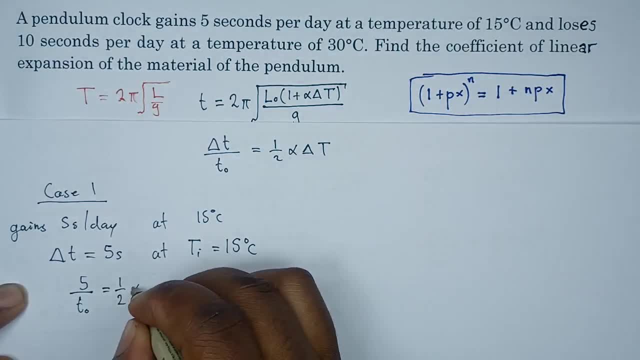 where it is alpha, we just have it as alpha. then the change in temperature. remember, change in temperature is T final minus T initial. we have the initial temperature, so T final minus the initial temperature that we have. so let's just put T sub f. initial is 15, so we can just refer to this as equation 1 and come back to it. 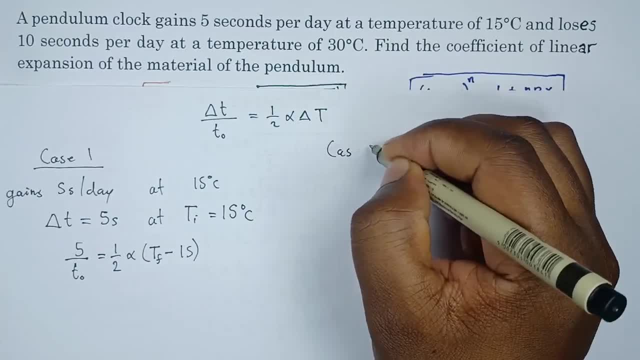 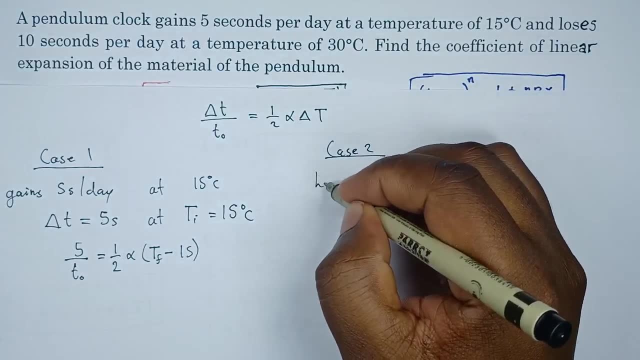 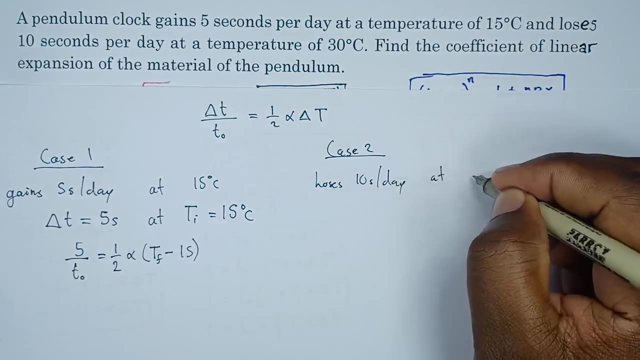 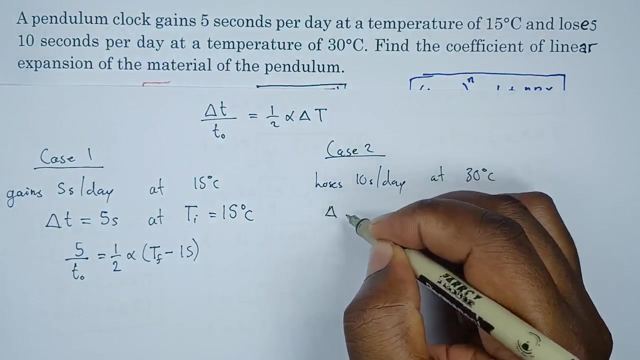 the second part, which is case 2, we have been told that it loses 10 seconds per day. so loses 10 seconds per day at a temperature of 30 degrees Celsius. what does this mean for us? so the change in temperature will be 10 seconds, sorry a. 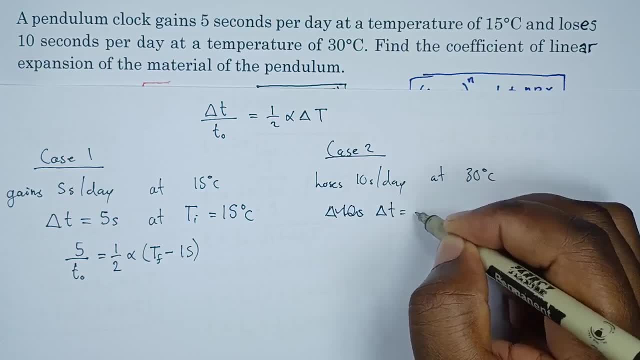 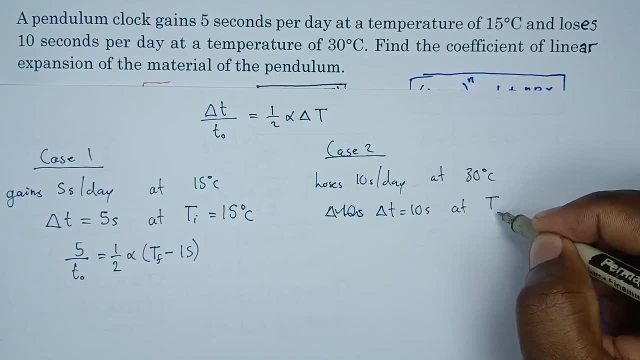 change in time. change in time will be 10 at the temperature. now, this temperature that we have here is the final temperature, 30 degrees Celsius, remember. but this one is losing the other one's game. the idea is the final temperature, or case one that was the initial final temperature, for case one becomes the 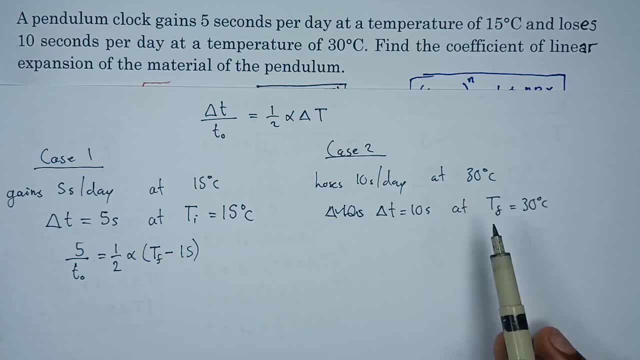 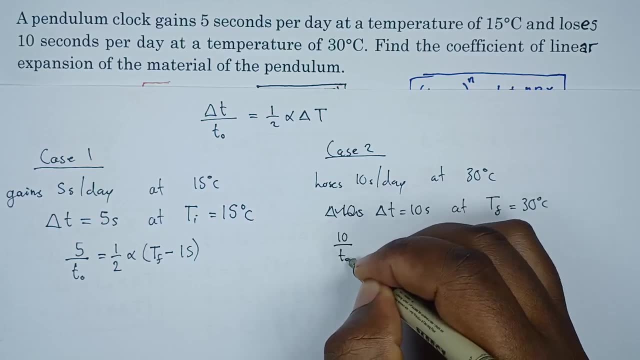 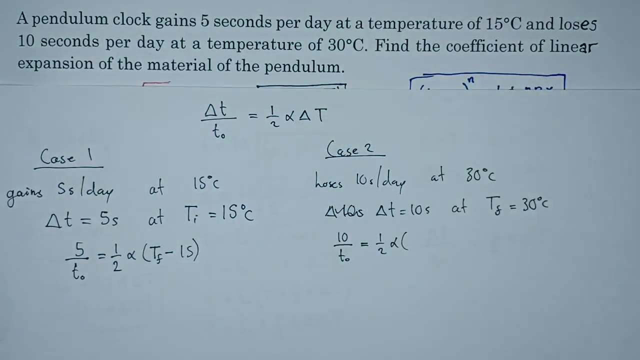 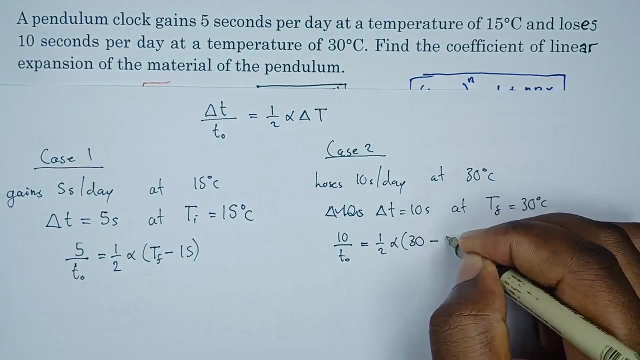 initial temperature, or case two, so on. this expression now let's substitute in our formula: change in time is 10 over T naught, as opposed to half alpha. now, changing temperature, it's final minus initial, but this time around we are saying that the final we have is 30. what we don't 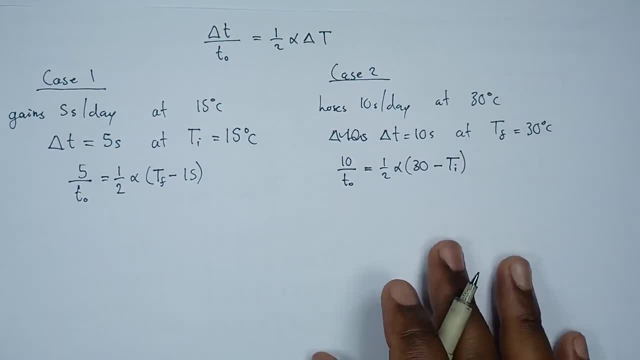 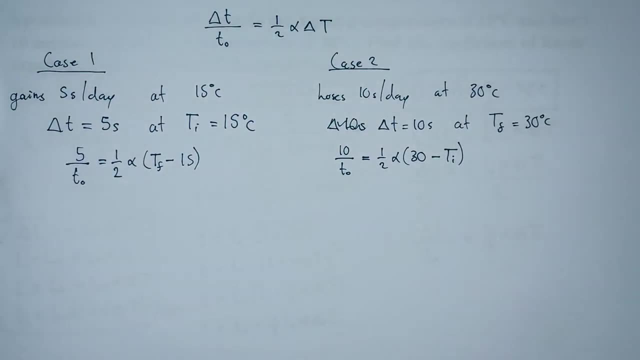 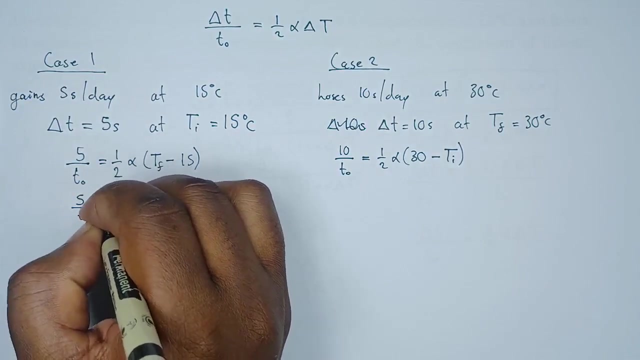 have is the initial. now remember what I've just said: the final temperature in case one is the initial temperature in case two. so we can write these two by simply saying: five over t naught is equal to half alpha, so instead of T final, let's just call it T. 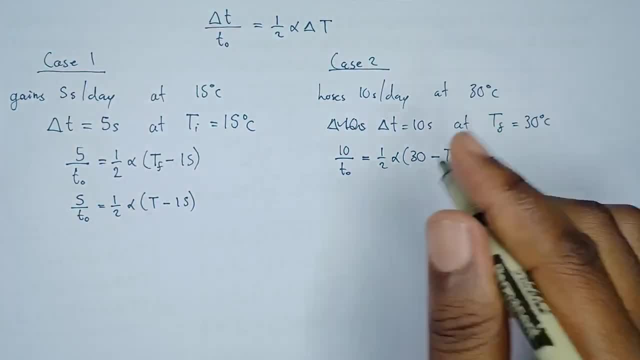 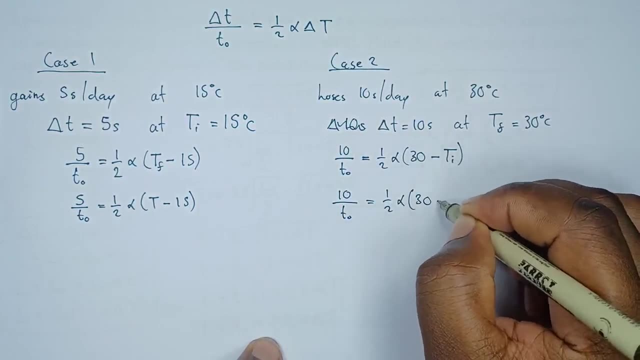 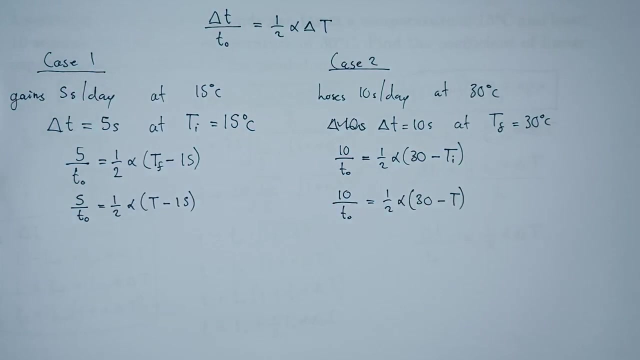 it's the same as the other temperature we have here. so 10 over T naught is equal to half alpha T minus T. why is it the same T? like I said, final in case 1 is equal to initial in case 2. what we want to do is we combine these two equations. I'll divide this one by: 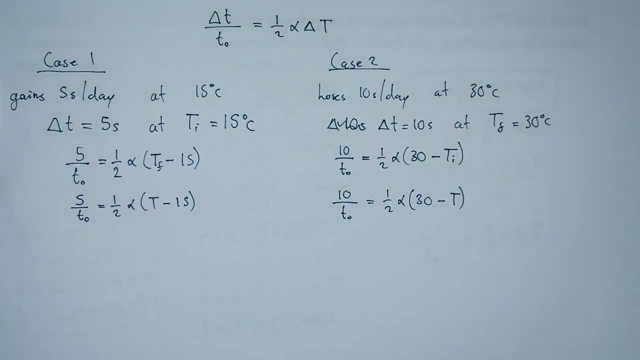 over this one. so dividing case one equation over case two. so we're going to get on the left hand side. we divide these two so we have five t naught divided by this expression, which is 10 t naught is equals to same thing. on this side. we divide this over that. what we get, we get. 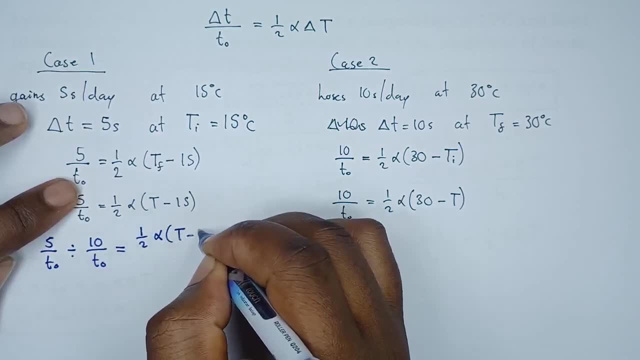 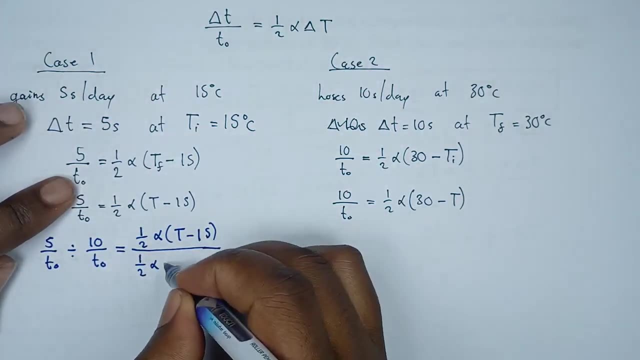 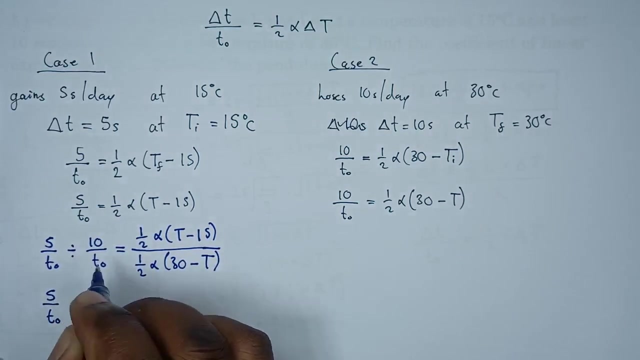 half alpha t minus 15 divided by this, which is half alpha 30 minus t, like that. so the moment we do that on the left hand side in this part here, we're going to have 5 over t naught multiplied by the reciprocal, which is t naught over 10. 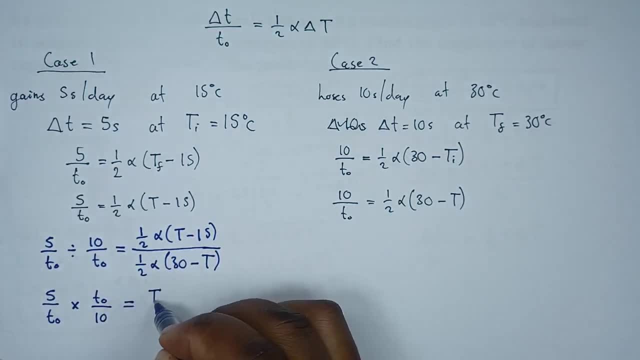 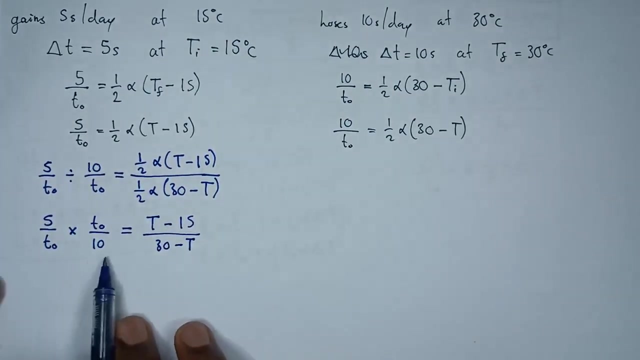 the half of cancel, the alpha of cancel. we want to remain with t minus 15 over 30 minus t, like that. so what do we obtain here? in this part, we can see that the t naught will cancel out, giving us with 5 over 10. now, 5 over 10 is just as good as 1 over 2. 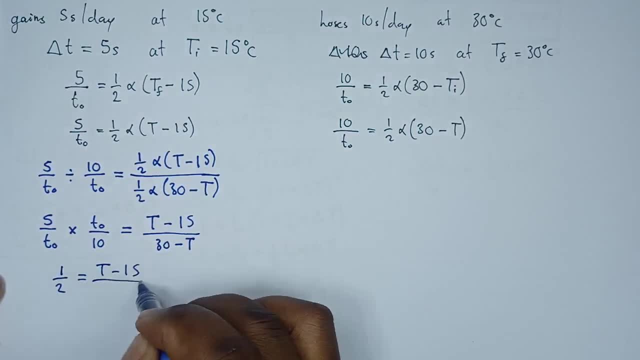 reduce it. this equals to t minus 15 over 30 minus 15 over 30 minus t. we can cross, multiply so that we get t minus. let me say two t, so two times t. so two t minus thirty is equals to thirty minus t. so we have that. so let's put the t on one side and 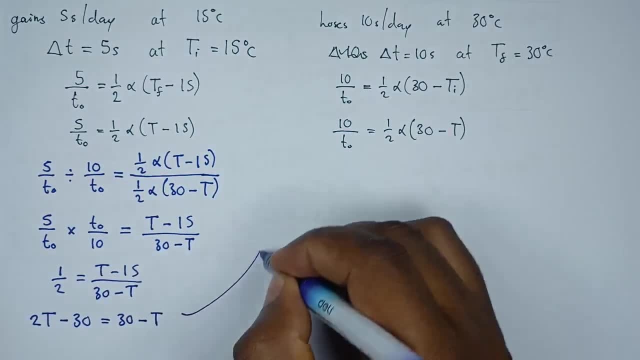 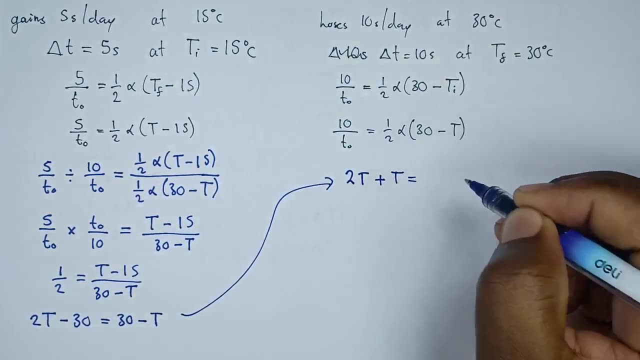 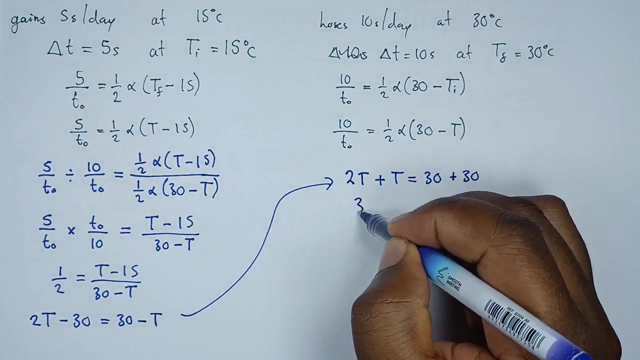 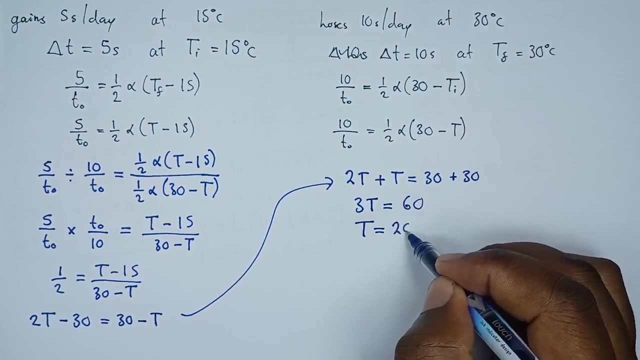 everything else on the other side, what we're getting here, let's just bring here. what we're getting here will be: 2t plus t is equals to 30. this negative 30 will cross the cosine to become a positive 30. so 3t is equals to 2kst, knowing that t is simply 20.. now remember, t is temperature. 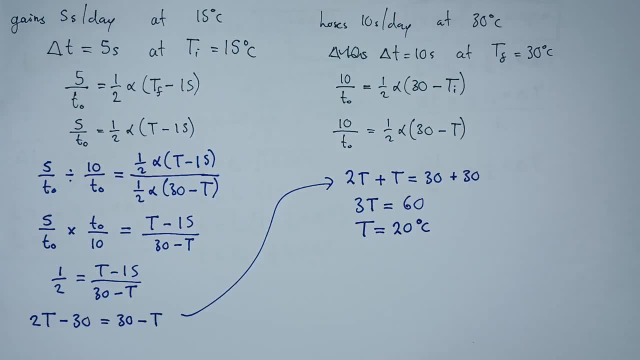 so 20 degrees celsius. so now that we have the 20, remember our goal is to find alpha. so, to find alpha, what i want to do, i want to choose one of the equations that we can use. let's use equation one, for example. so this equation from case one, you can use this one as well. 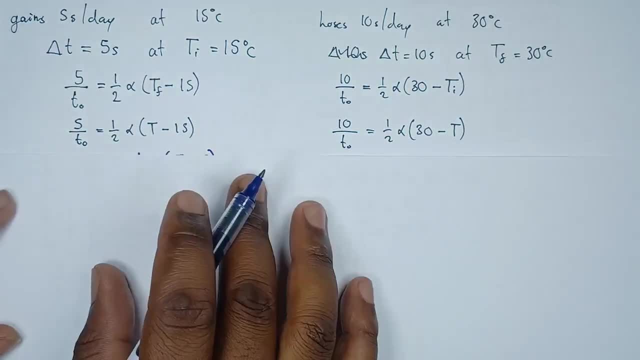 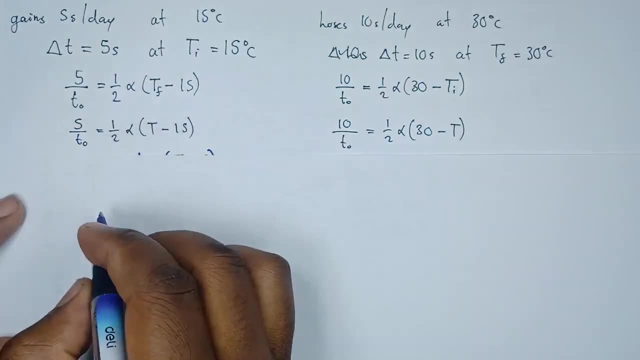 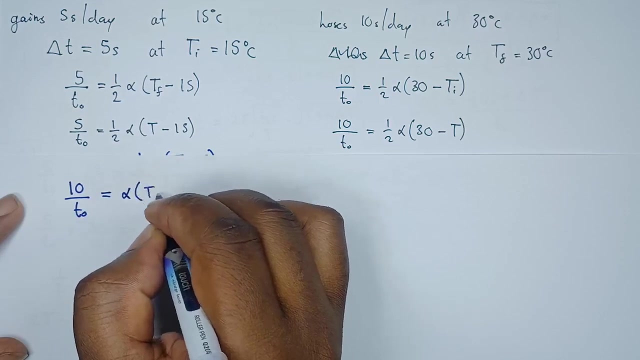 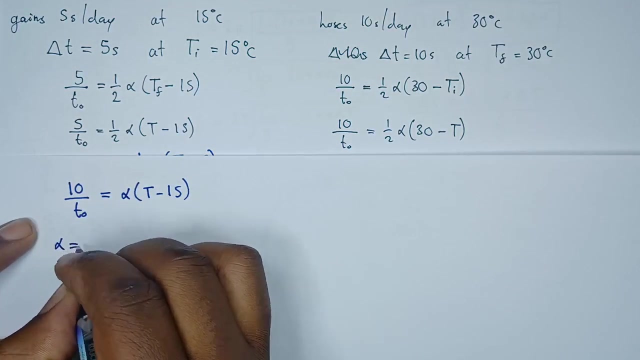 either way, it's okay, i'll look for alpha, remember. so let's make alpha the subject of formula. so if we cross, multiply these two multiply five, hence we get 10 over t naught is equals to alpha t minus 15.. we divide both sides by t minus 15, hence alpha is equals to 10 over t naught, t minus 15.. now 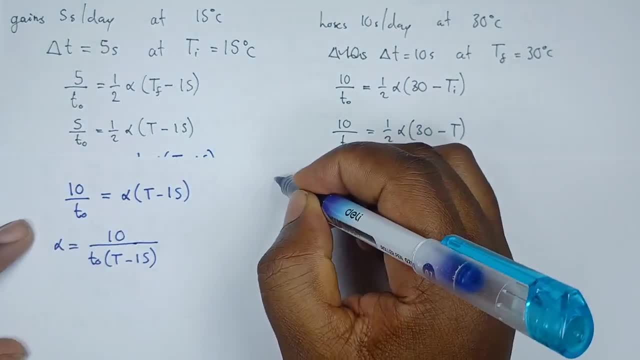 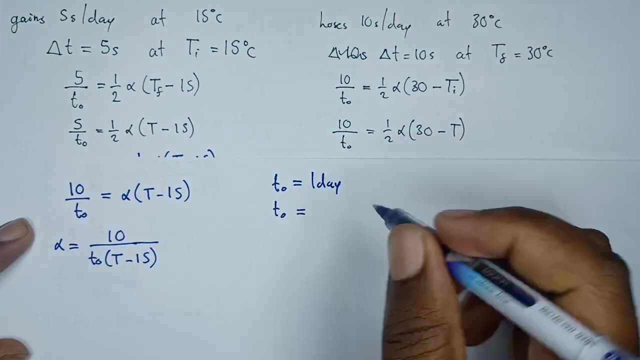 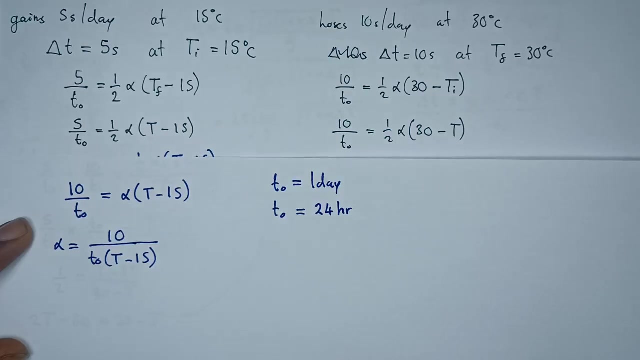 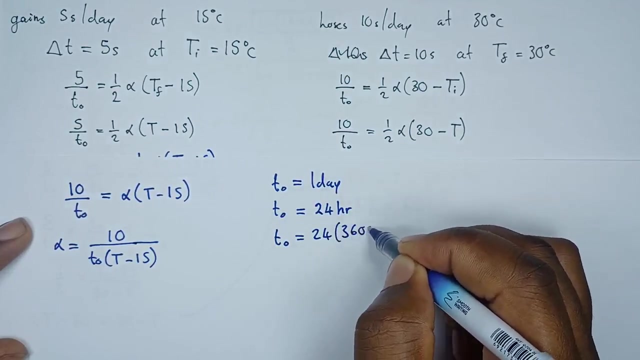 this time change was per day, so remember the initial time we're going to say. since it's for one particular day, then t initial will be remember. in a day there are 24 hours now, in an hour, in an hour, there is 3600 seconds, knowing that t initial is 86.